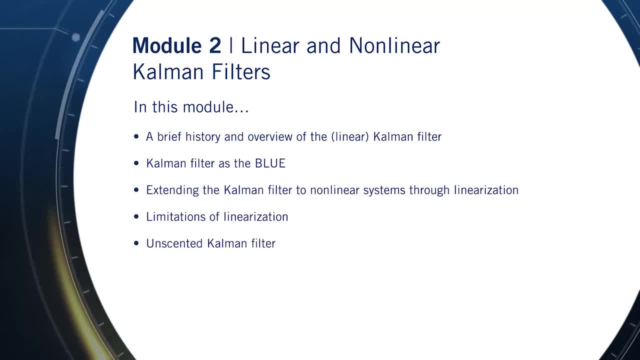 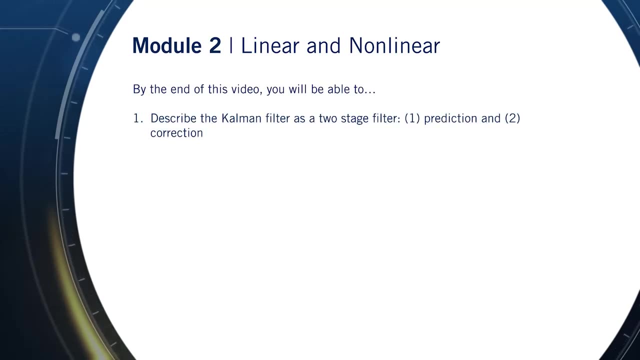 Discuss limitations of this linearization approach and finally present a modern alternative to linearization through the unscented transform. By the end of this lesson, you'll have learned a lot. You'll be able to describe the Kalman filter as a state estimator that works in two stages- prediction and correction- understand the difference between motion and measurement models. 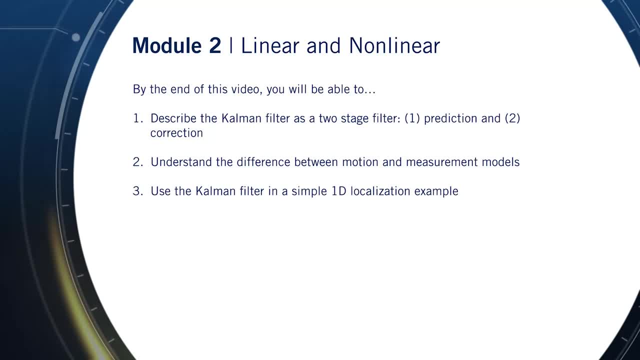 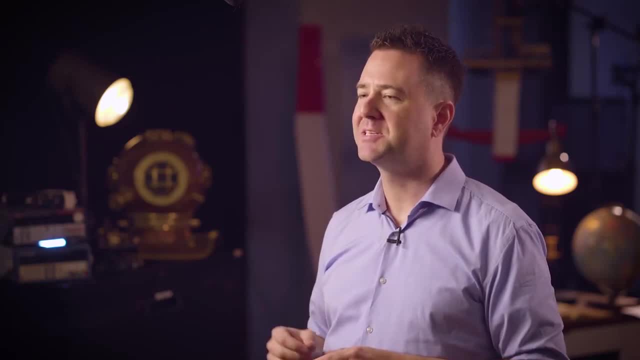 and then use the Kalman filter formulation in a simple 1D localization example. Let's begin with a bit of history. The Kalman filter algorithm was published in 1960 by Rudolf E Kalman, a Hungarian-born professor and engineer. 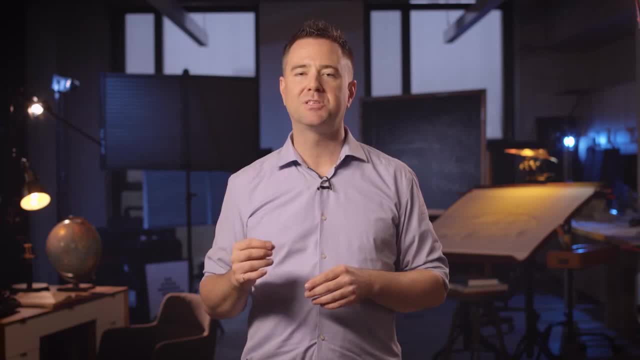 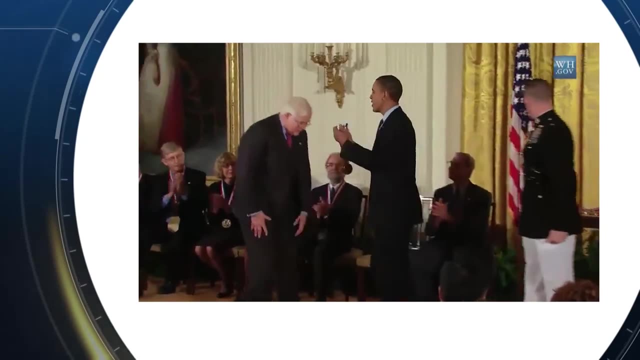 who was working on the Kalman filter. He was working at the Research Institute for Advanced Studies in Baltimore, Maryland. Years later, in 2009,. American President Barack Obama awarded Kalman the prestigious National Medal of Science for his work on the Kalman filter. 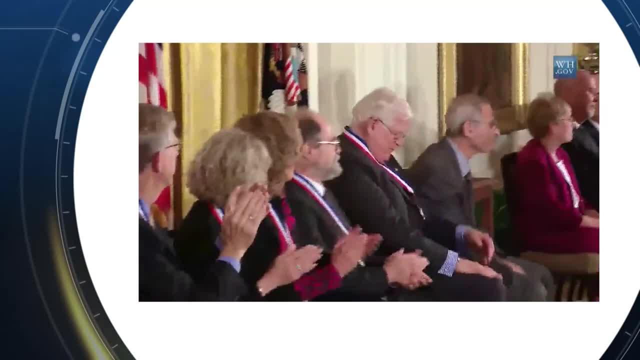 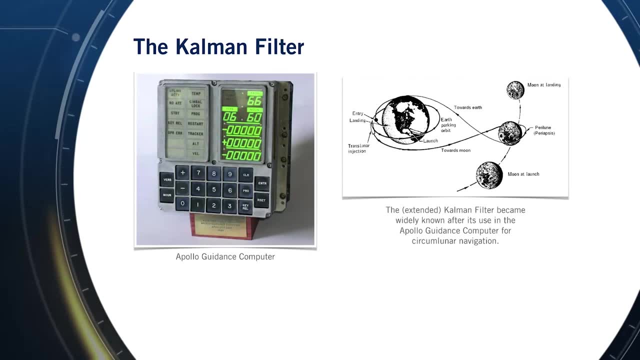 and other contributions to the field of control engineering. After its publication in 1960, the Kalman filter was adopted by NASA for use in the Apollo guidance computer. It was this groundbreaking innovation that played a pivotal role in the development of the Kalman filter. 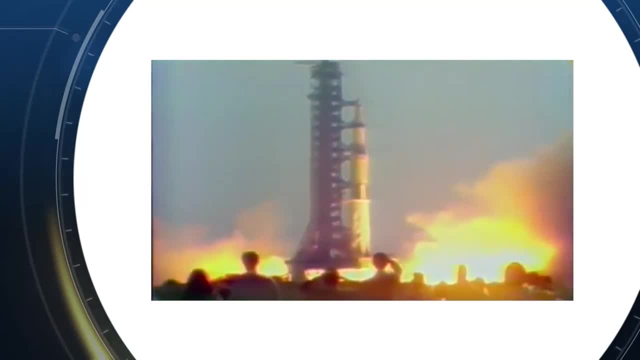 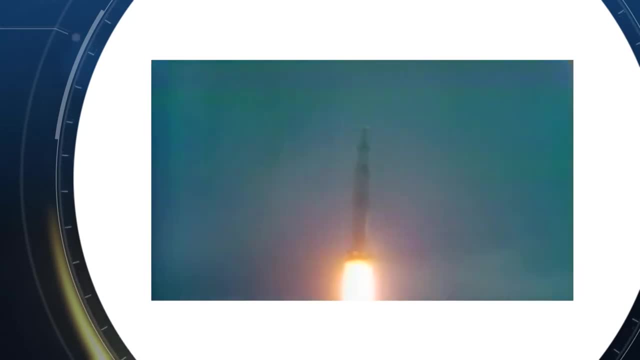 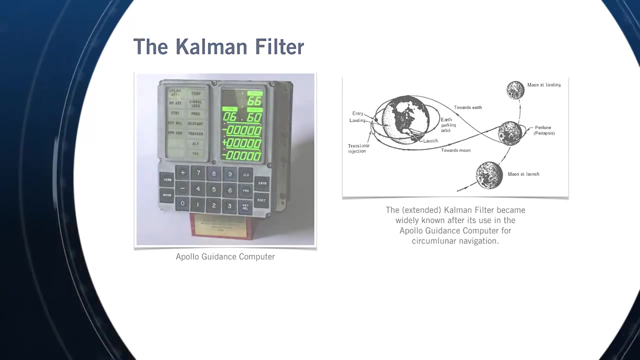 The experiment played a pivotal role in successfully getting the Apollo spacecraft to the Moon and to our first steps on another world. The filter helped guide the Apollo spacecraft accurately through its circumlunar orbit. The engineers at NASA's Ames Research Center adopted Kalman's linear theory and extended it to non-linear models. 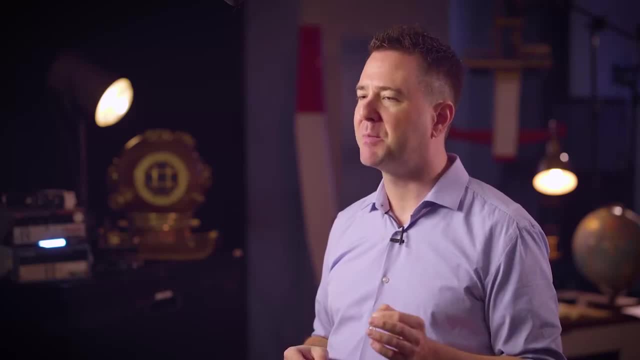 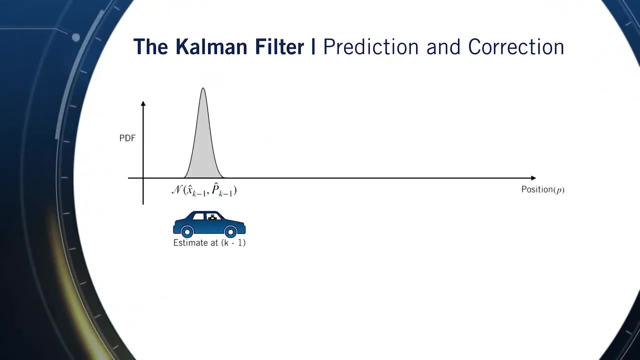 We'll look at this specific extension in an upcoming module, But first let's talk about the basic linear Kalman filter. The Kalman filter is very similar to the linear recursive least squares filter we discussed earlier. While recursive least squares updates the estimate of a static parameter, 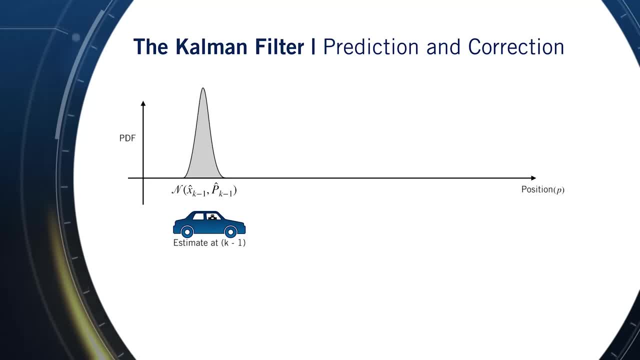 the Kalman filter is able to update an estimate of an evolving state. The goal of the Kalman filter is to take a probabilistic estimate of this state and update it in real time using two steps: prediction and correction. To make these ideas more concrete, let's consider a problem of estimating the 1D position of a vehicle. 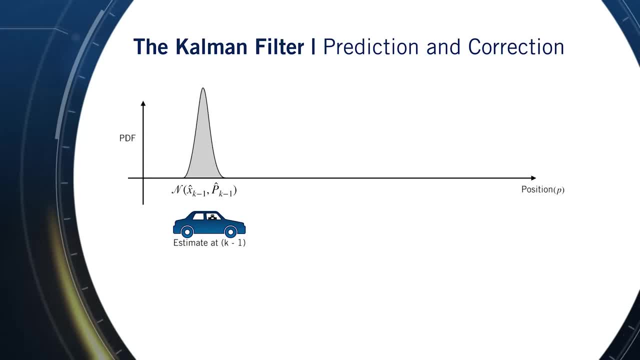 Starting from an initial probabilistic estimate at time k-1,, our goal is to use a motion model which could be derived from wheel odometry or inertial sensor measurements to predict our new state. Then we'll use an observation model derived from GPS, for example. 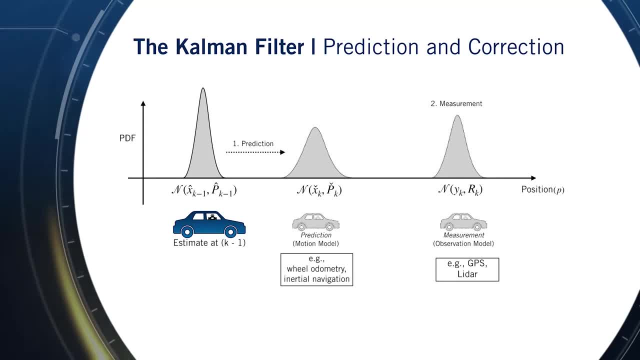 to correct the 1D position of a vehicle, To correct that prediction of vehicle position at time k. Each of these components- the initial estimate, the predicted state and the final corrected state- are all random variables that we will specify by their means and covariances. 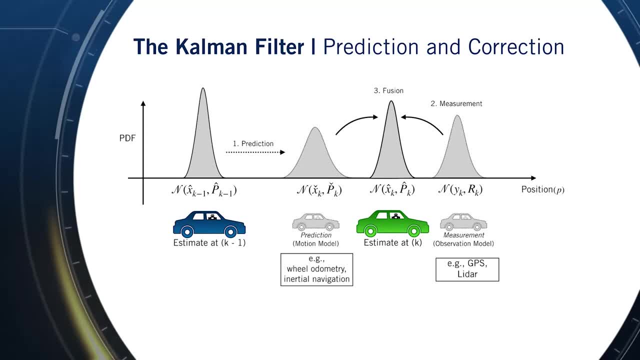 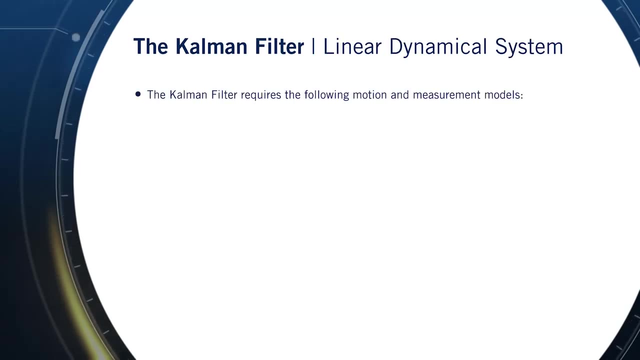 In this way, we can think of the Kalman filter as a technique to fuse information from different sensors to produce a final estimate of some unknown state. taking into account uncertainty in motion and in our measurements For the Kalman filter algorithm, we have been able to write the motion model in the following way. 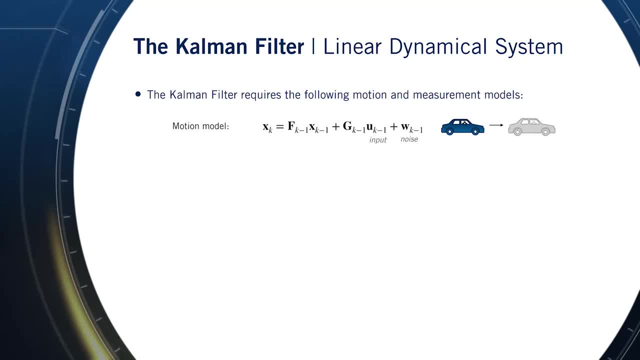 The estimate at time step k is a linear combination of the estimate at time step k-1, a control input and some zero mean noise. The input is an external signal that affects the evolution of our system state. In the context of self-driving vehicles, this may be a wheel torque applied to speed up and change lanes, for example. 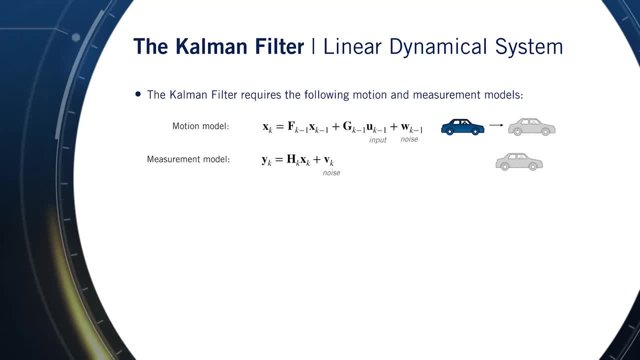 Next, we will also need to define a linear measurement model And, finally, we'll need a measurement noise, as before, and a process noise that governs how certain we are that our linear dynamical system is actually correct or, equivalently, how uncertain we are about the effects of our control inputs. 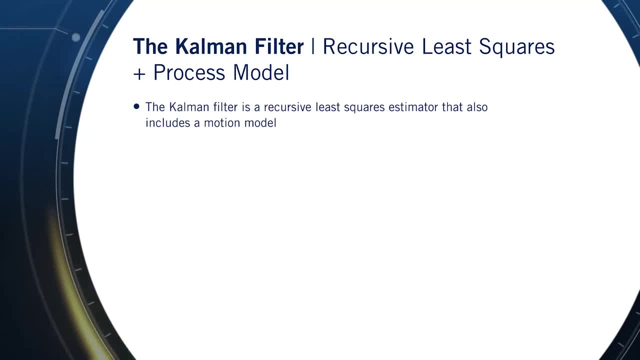 Once we have our system in hand, we can use an approach very similar to that we discussed in the recursive least squares video, except this time we'll do it in two steps. First, we'll use the process model to predict how our states –remember that we're now typically talking about evolving states and not state parameters– 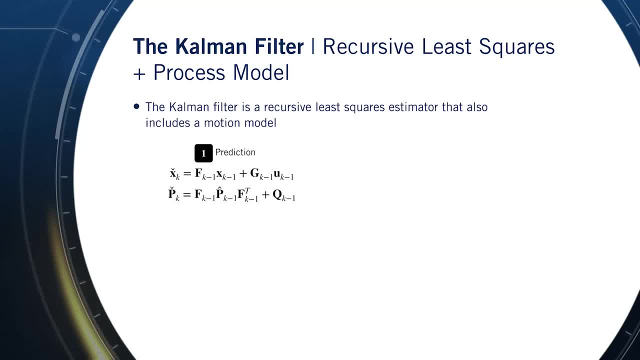 evolved since the last time step and will propagate our uncertainty. Second, we'll use our measurement to correct that prediction based on our measurement residual and our optimal gain. Finally, we'll use the gain to also propagate state covariance from our prediction to our corrected estimate. 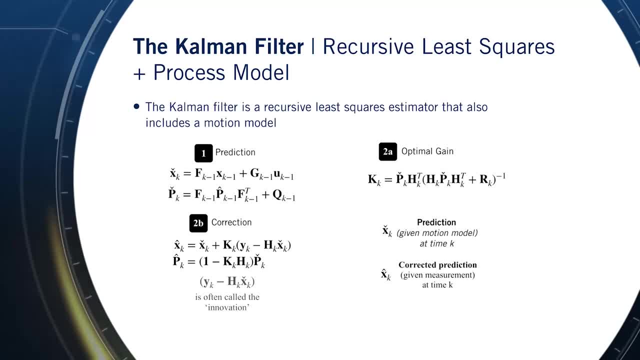 In our notation, the hat indicates a corrected prediction at a particular time step, whereas a check indicates a prediction before the measurement is incorporated. If you've worked with the Kalman filter before, you may also have seen this written with plus and minus signs. 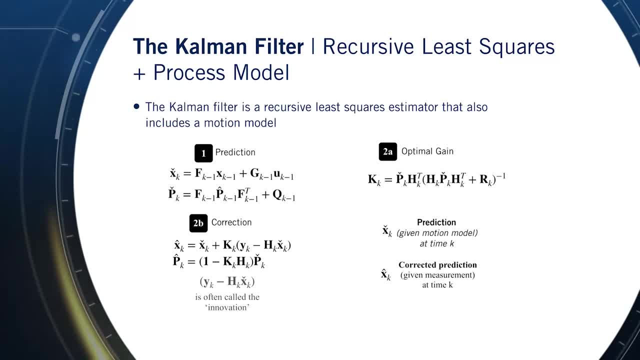 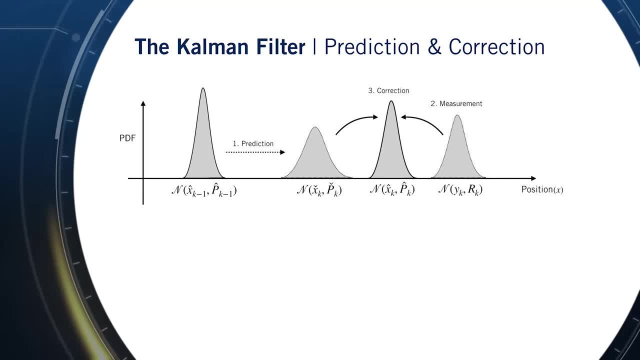 for the corrected and predicted quantities respectively. Let's recap: We start with a probability density over our states and also maybe parameters at time- step k minus 1, which we represent as a multivariate Gaussian. We then predict the states at time- step k using our linear prediction model. 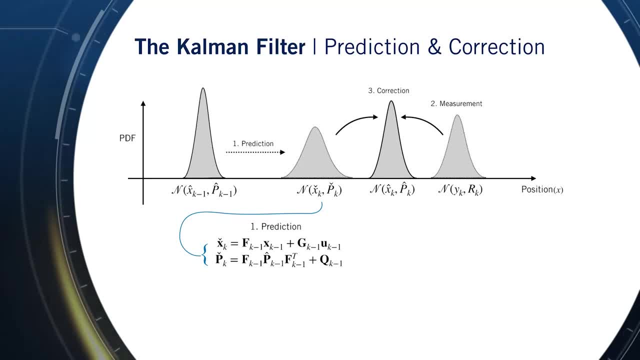 and propagate both the mean and the uncertainty, the covariance, forward in time. Finally, using our probabilistic measurement model, we correct our initial prediction by optimally fusing the information from our measurement together with the prior prediction through our optimal gain matrix k. 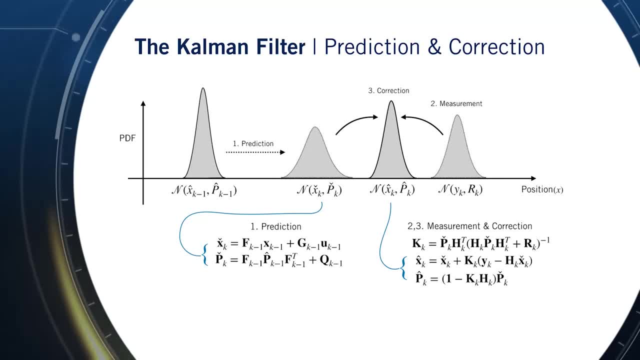 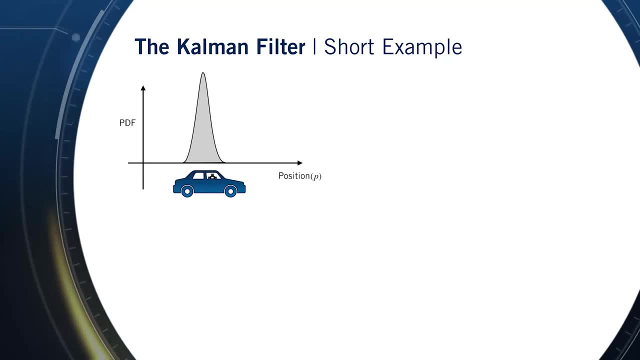 Our end result is an updated probabilistic estimate for our states at time. step k: The best way to become comfortable with the Kalman filter is to use it. Let's look at a simple example. Consider again the case of a self-driving vehicle estimating its own position. 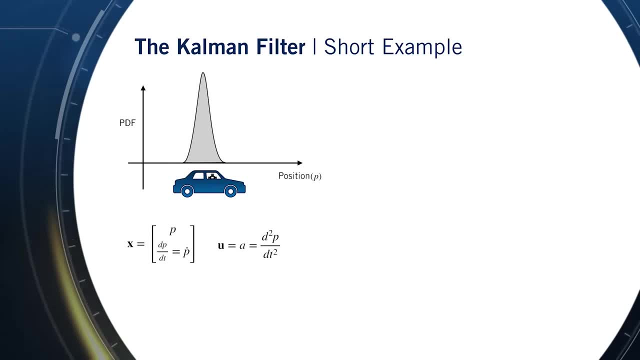 Our state vector will include the vehicle position and its first derivative velocity. Our input will be a scalar value, a scalar acceleration that could come from a control system that commands our car to accelerate forward or backwards. For our measurement, we'll assume that we're able. 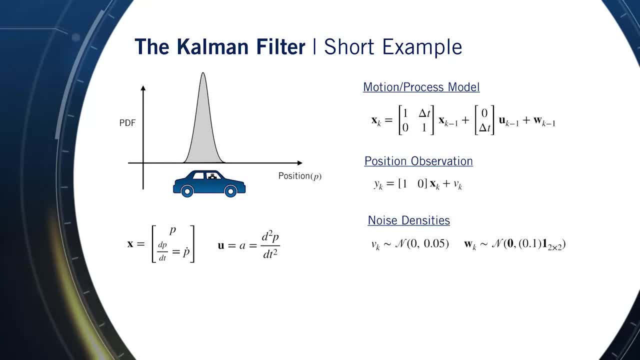 to determine the vehicle position directly using something like a GPS receiver. Finally, we'll define our noise variances as follows: Given this initial estimate and our data, what is our corrected position estimate after we perform one prediction step and one correction step using the data? 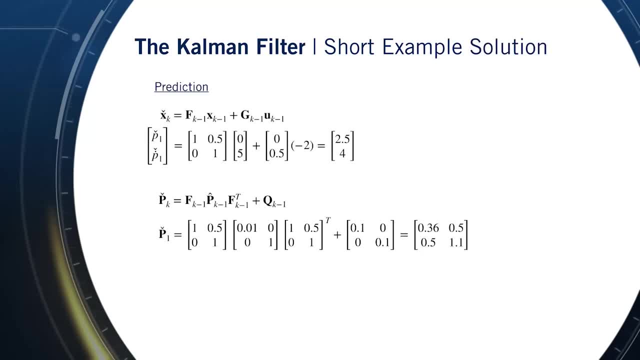 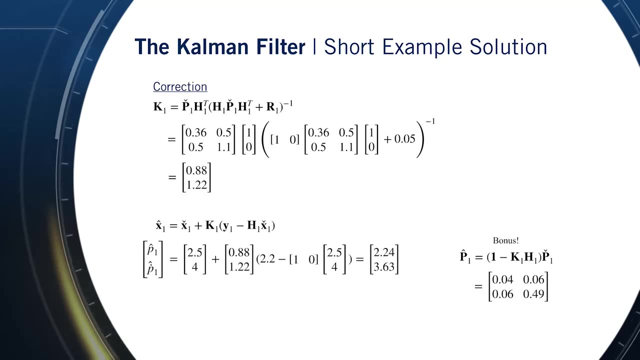 The almost always incorrect way to do this is by using the Kalman filter. Here is how we can use these definitions to solve for our corrected position and velocity estimates. Pay attention to the fact that our final corrected state covariance is smaller, That is, we are more certain about the car's position after we incorporate the position.